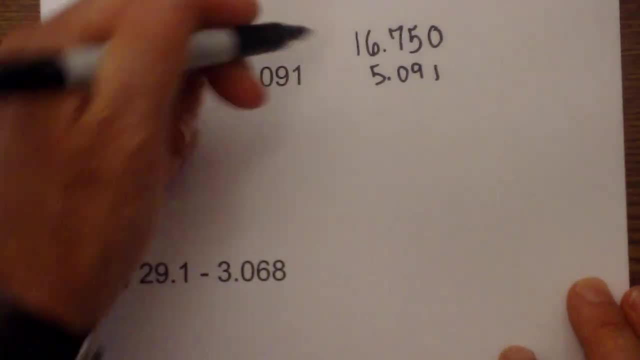 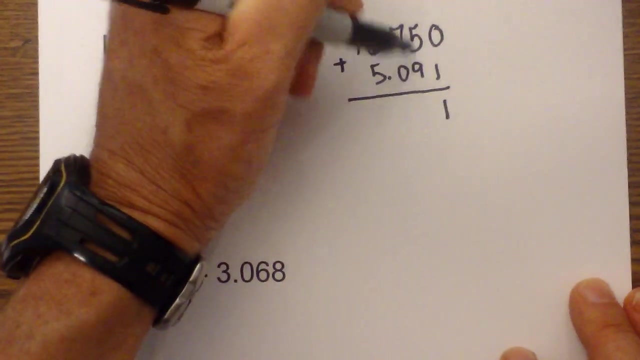 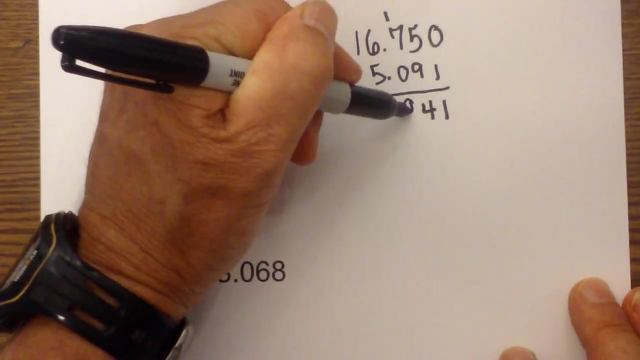 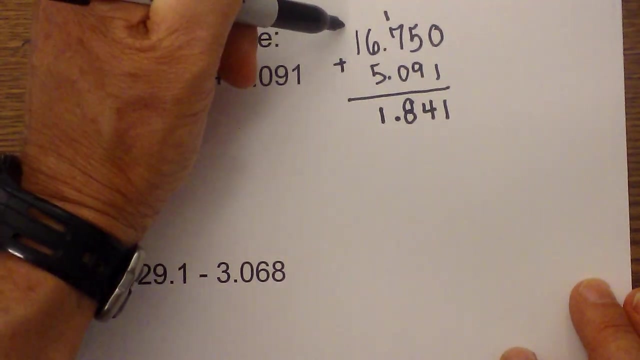 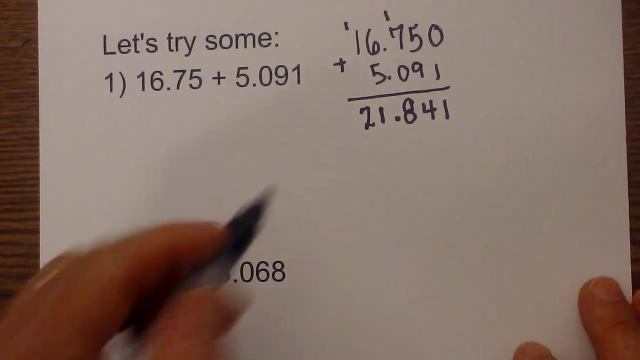 here as a placeholder to make it a little easier to see. Now this is subtracting. Excuse me. This is addition. So I just merely add 1 plus 0 is 1. 9 plus 5 is 14. Remember to carry the 1. 7 plus 1 is 8. Bring down the decimal. Okay. 6 plus 5 is 1. Carry the 10 over. Actually, it's 11. Carry the 10 over. So that becomes 21.84. Notice I lined up the decimals and then just 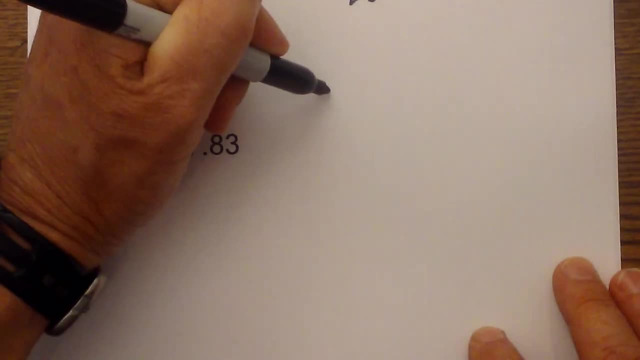 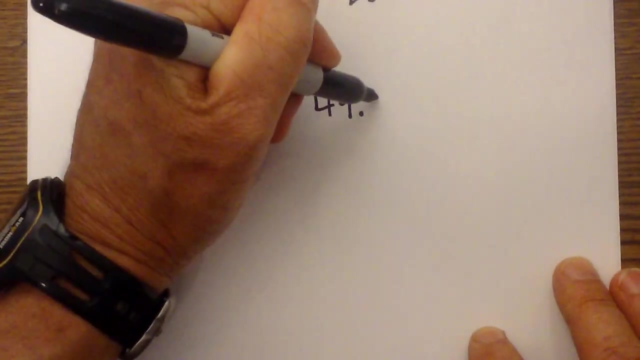 merely add. Let's go ahead and look at another addition. 49. And I'm going to go ahead and write a decimal there because we know any number where there's not a decimal, it's always at the end. 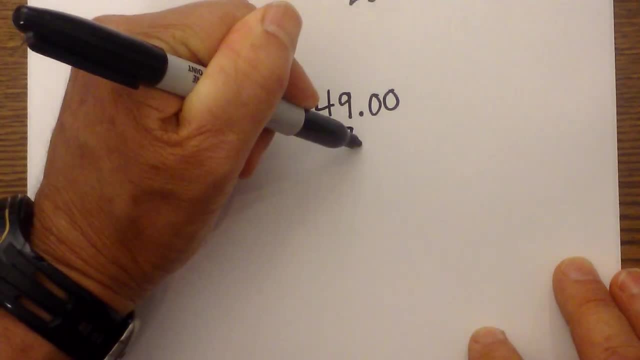 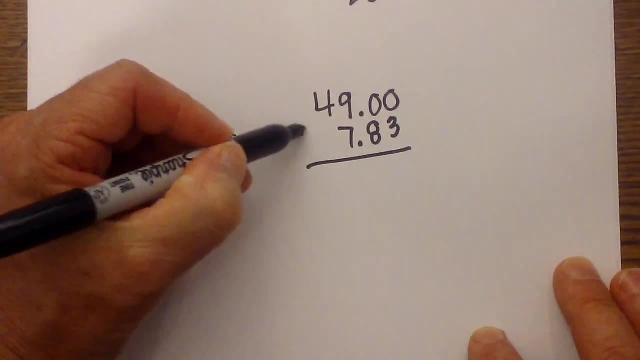 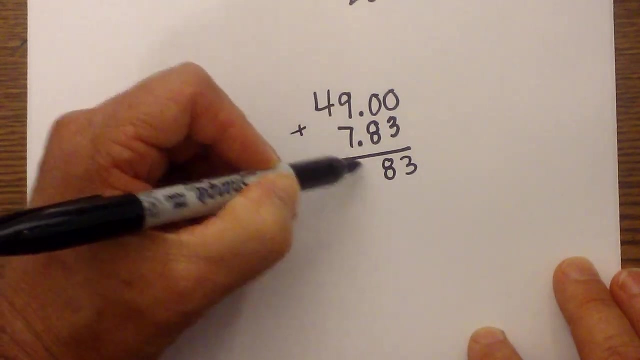 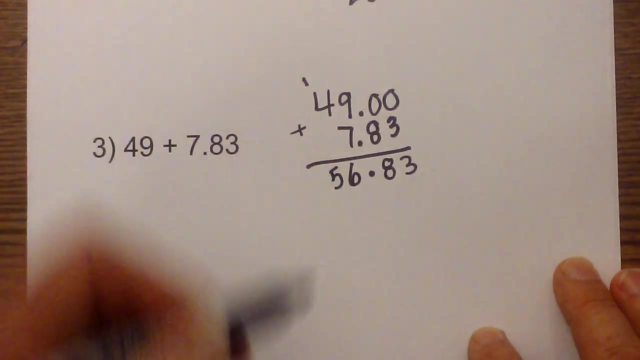 And I'm going to add a couple of zeros. And then we have 0, excuse me, 7.83. Notice that the decimals are lined up. Now we just, this is addition. So I'm just going to add 3 plus 0 is 3. 8 plus 0 is 8. 9 plus 7. Bring down the decimal. 9 plus 7 is 16. Carry the 1. 4 plus 1 is 5. So that is 56.83. Now let's get to a couple of 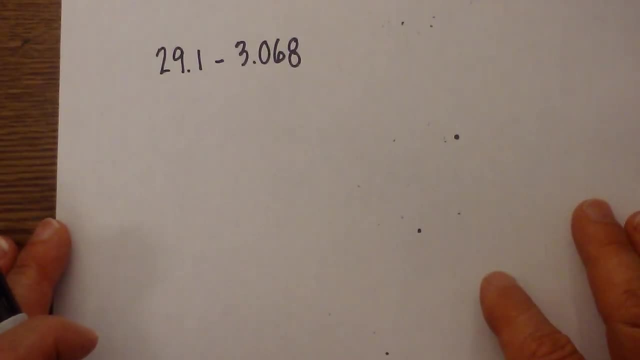 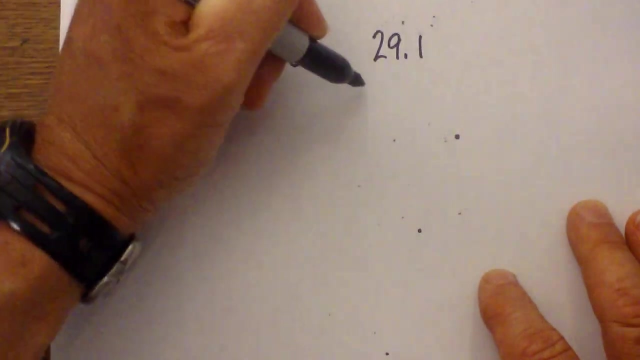 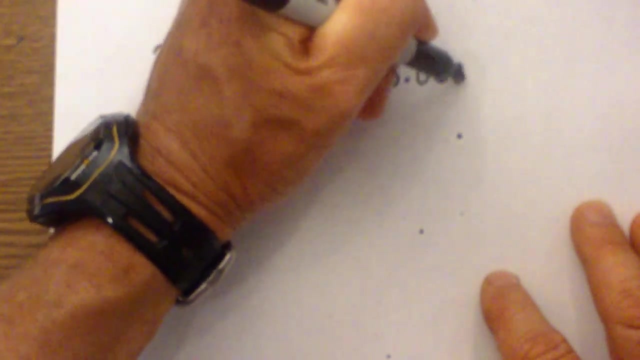 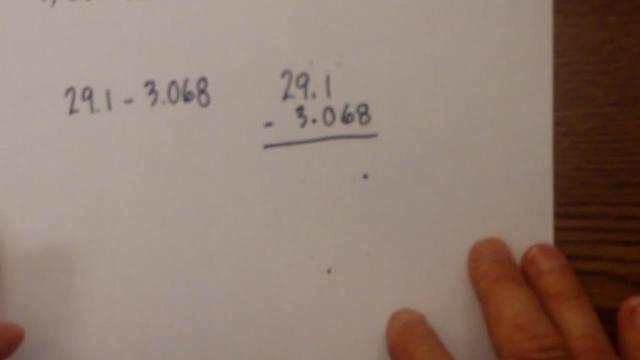 subtraction problems. Okay. Why don't I go ahead and work this one first. 29.1 minus 3.068. I'm going to rewrite the 29.1 minus 3. Notice I've lined up the decimal 068. And you can see this will get a little bit easier to subtract. So I'm adding this one up. So a couple of zeros to make that a little bit easier to subtract. So I'm adding zero. Now we have 8 minus zero. So if 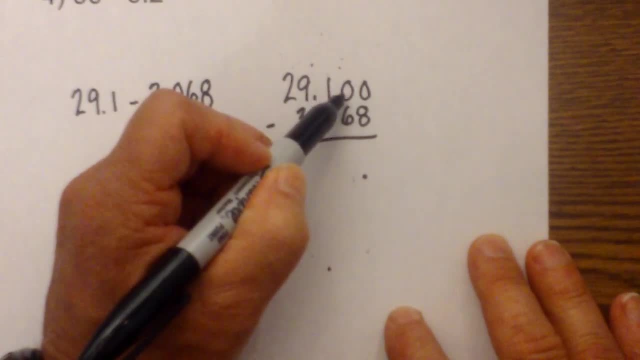 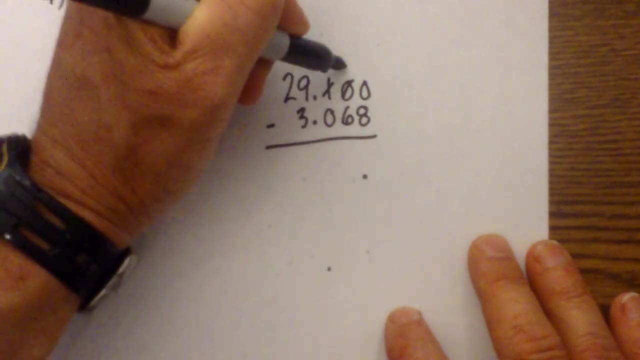 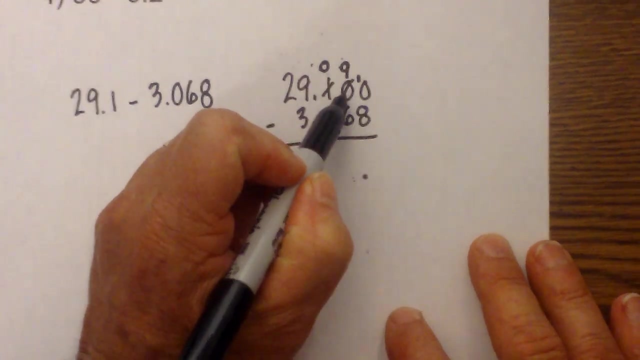 it's a minus zero, it can't borrow 1 from next door because it's a zero. So we have to borrow it from the 1 way over here. So this becomes a zero. This will become a 9 because this zero needs to borrow one. Okay so you can't borrow from a zero if you don't have a zero. You can't borrow from a zero because there's seven zeros there. If you do, you will borrow from a 3. So that's 5.9. But one zero doesn't count. You didn't borrow from a zero unless all the zeros here are in union and you 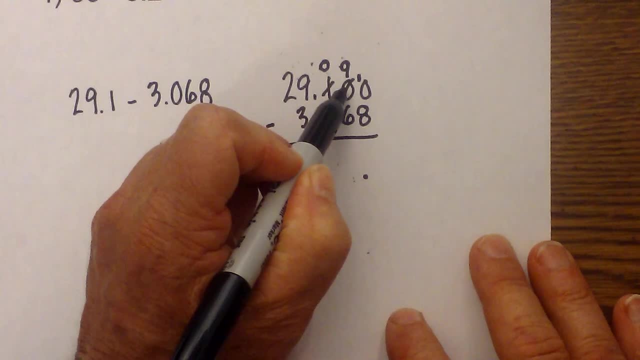 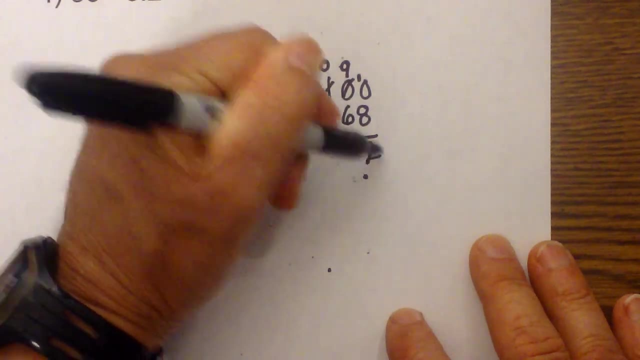 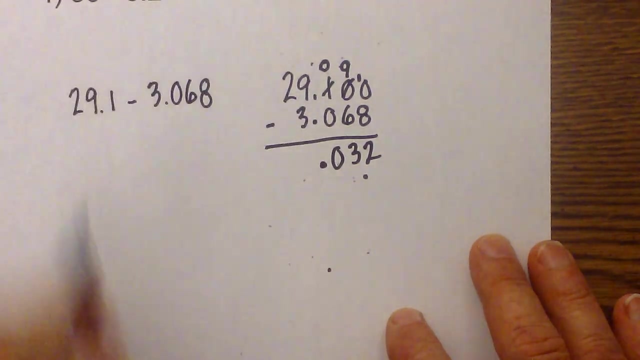 borrowed from the 1 and then this guy borrowed from this one so it becomes a 9 and that becomes a 10 now 8 excuse me 10 minus 8 is 2 9 minus 6 is 3 0 minus 0 is 0 bring down the decimal 9 minus 3 is 6 and we can bring down the 2 so we 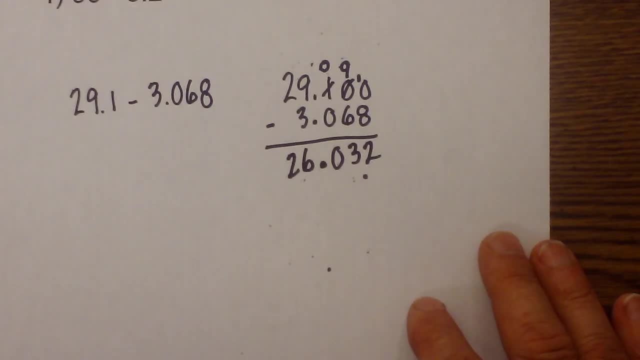 get 26 point 0 3 2 okay that's a little tricky just remember you cannot borrow 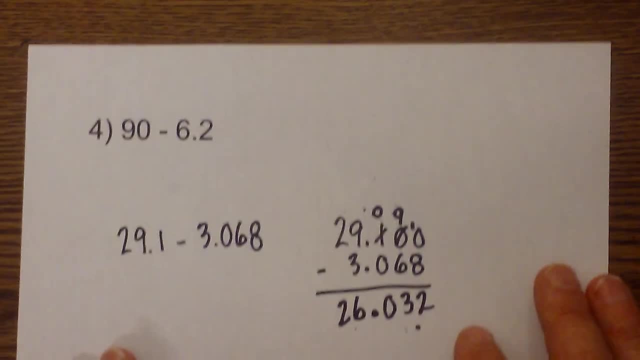 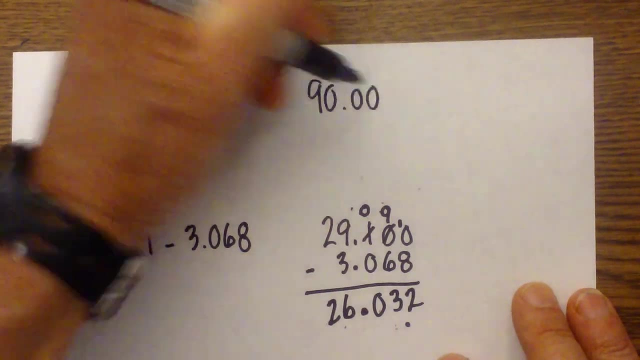 anything from the 0 okay and finally let's work one more example I'll rewrite this one 90 I'm gonna add a couple zeros at the end here's your decimal 6.2 okay 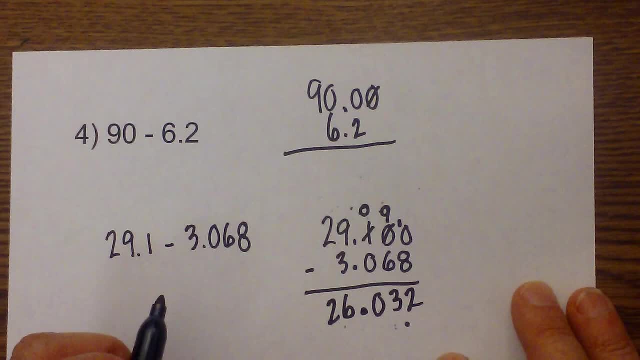 and I guess I really don't need that zero there okay okay okay 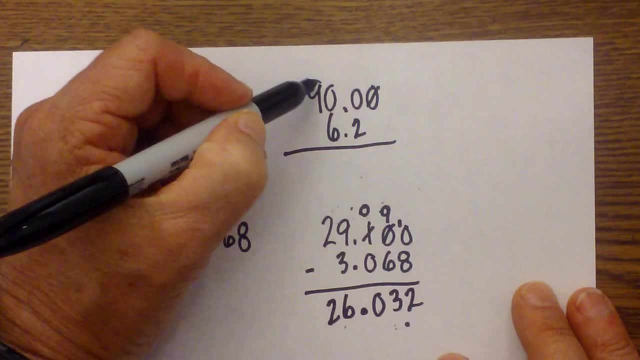 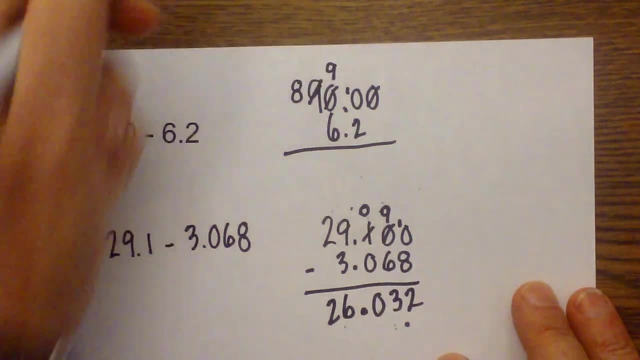 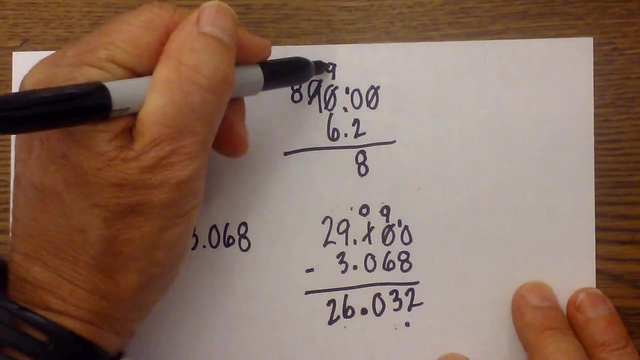 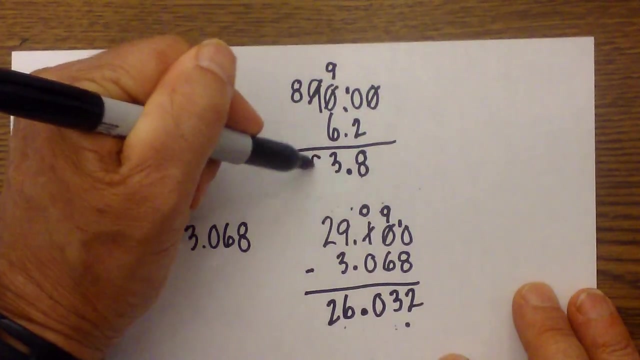 0 needs to borrow some from this 0 which can't do that so this is going to become an 8 this 0 will become a 9 and this will become a 10 okay 10 minus 2 is 8 9 minus 6 is 3 be careful bring down the decimal okay and then this is 8 so that becomes 83.8 okay 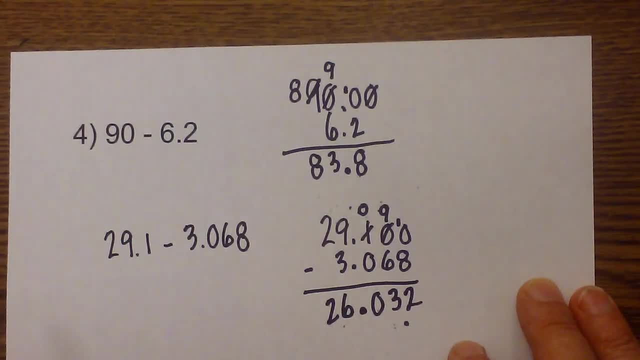 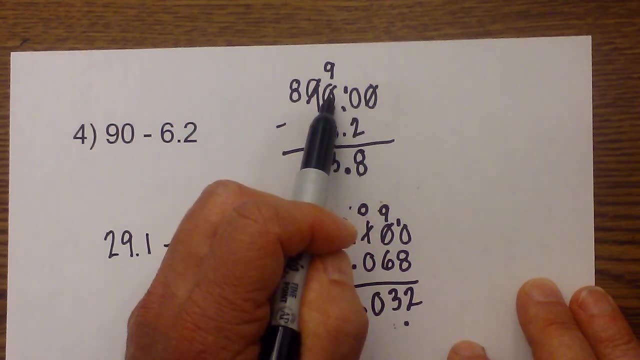 in summary remember always line up the decimals then you just subtract normally remember you cannot 0 you cannot borrow 1 from another 0 you have to move down the line and hope that helps with adding 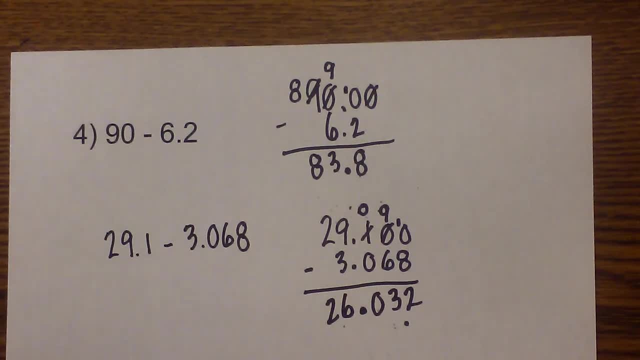 and subtracting decimals MooMooMath uploads a new math video every day thanks for watching